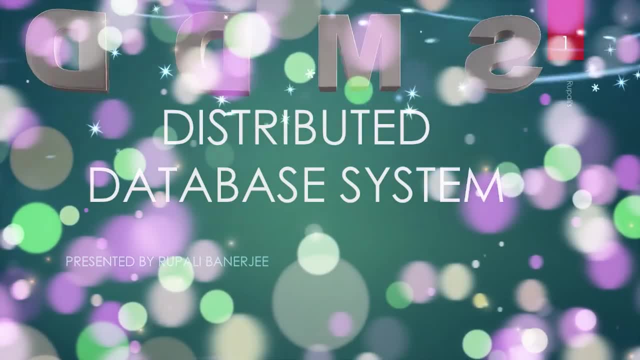 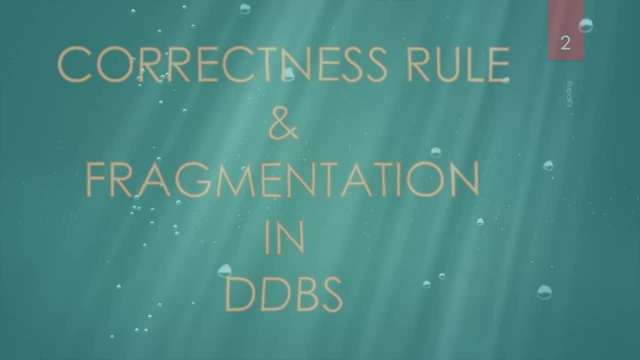 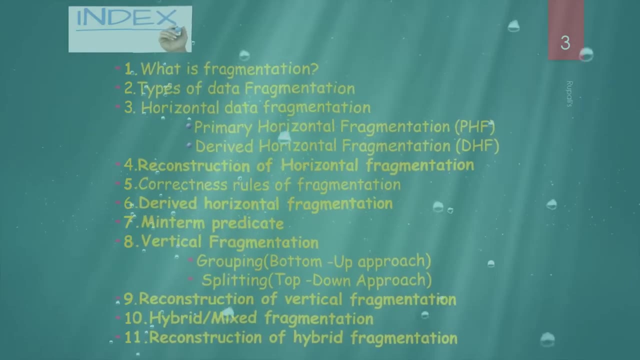 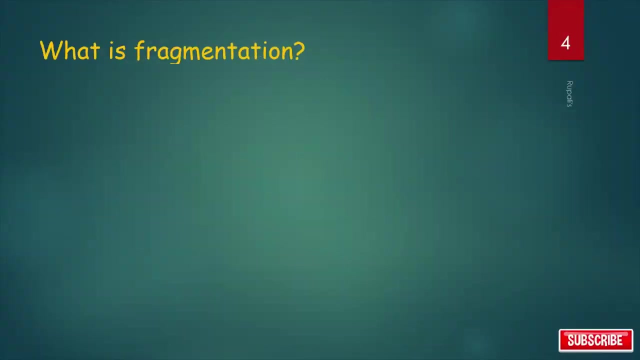 Distributed database system presented by Rupali Banerjee. So today our topic is correctness rule and fragmentation in distributed database system. Today we will going to cover following topics: See the index carefully. What is fragmentation In a distributed database system? the whole database is. 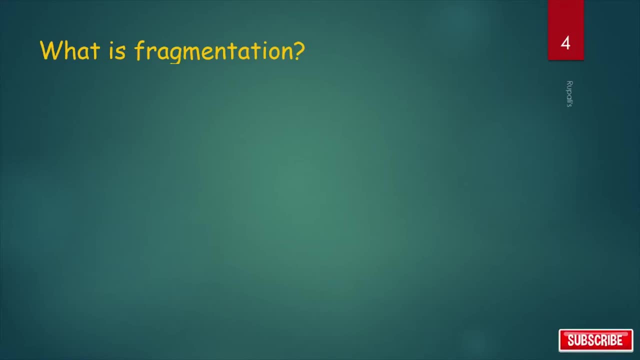 fragmented. Fragmented means what The whole database is divided in multiple parts and it is distributed in different sites. So what is fragmentation? The process of dividing the database into a smaller, multiple parts is called as fragmentation. Then these fragments may be stored at different locations or sites. The data fragmentation process should be carried out in. 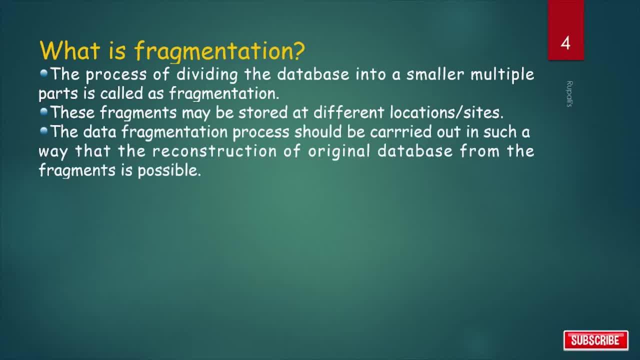 such a way that the reconstruction of the original database from the fragments is possible. If I want to reconstruct again the original database from the fragments, then it is possible. Types of data fragmentation. There are three types of data fragmentation. First one is horizontal data fragmentation. second one is vertical data fragmentation and third one is hybrid fragmentation. 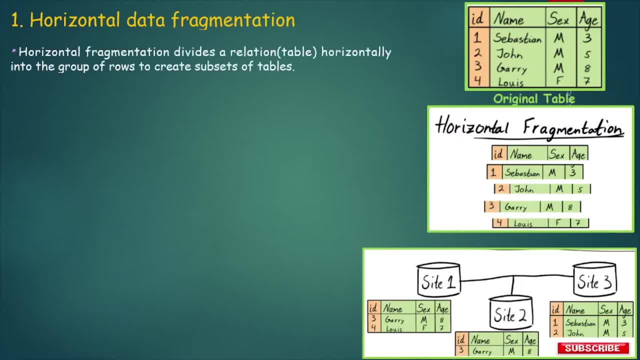 Horizontal data fragmentation. In case of horizontal data fragmentation, first it divides a relation or a table horizontally into a group of rows to create subset of the original table. In horizontal fragmentation, table is partitioned with respect to tuples. Tuples means rows. It breaks original relation r by assigning each tuple r to one or more fragments. Every fragment has 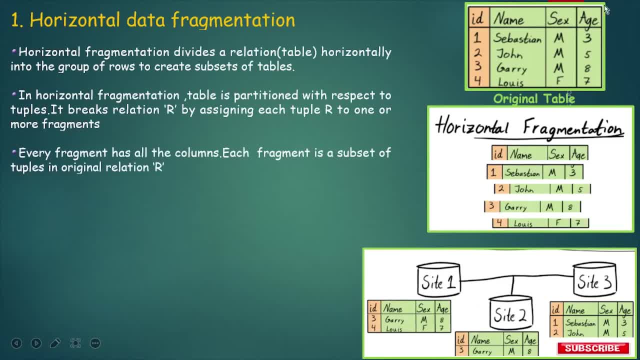 all the columns: See table. this original table has four columns, So every fragment has all four columns. Each fragment is a subset of tuples in original relation. Here you can see both columns are displayed in vertical order. in Gemeinscher says אםürk Protein and w empirics says attraction are all fragments are stored at different sites. 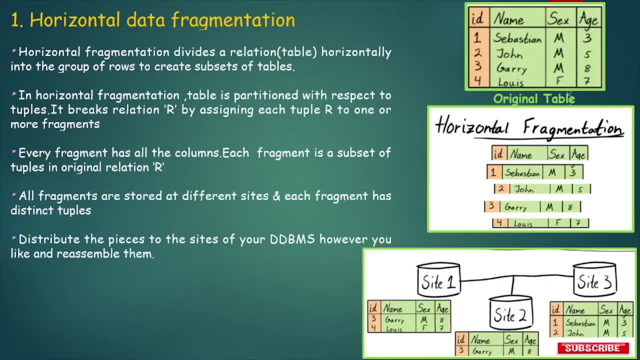 see, it stores a different file. It is found that each fragment has distinct tuples. Distribute the pieces to the sides of your distributed database management system, however you like, and reassemble them. If I want to reassemble these fragments, we can get the original table. There are two types of horizontal data fragmentation. one is primary. 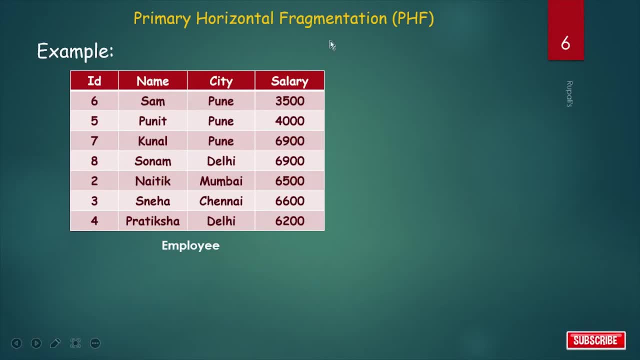 write horizontal fragmentation. take one example, then this thing will be more clear for you. primary horizontal fragmentation: this is one table of employee and the columns are id name, city and salary. now i have to create fragments based on city. fragment one is i have to select those employee. 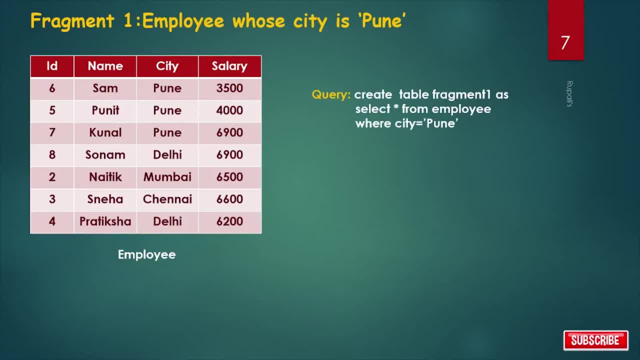 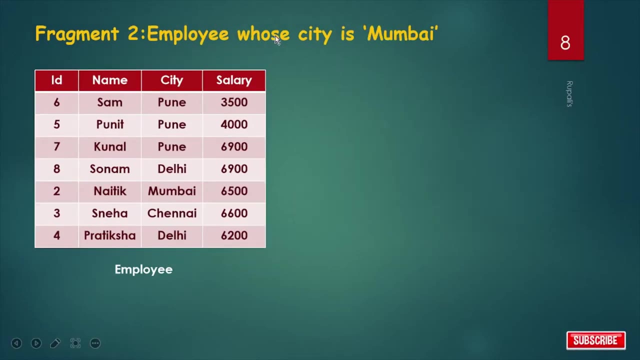 whose city is pune. so what should be the query? query is like this: create table fragment one as select star from employee where city equals to pune. so fragment one will be like this. in the same way, for fragment two, i have to select those employee whose city is mumbai. so query: 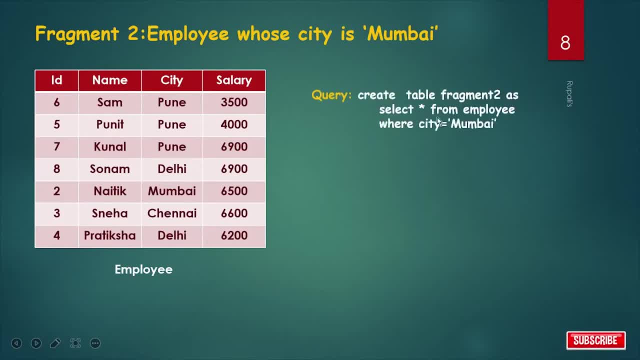 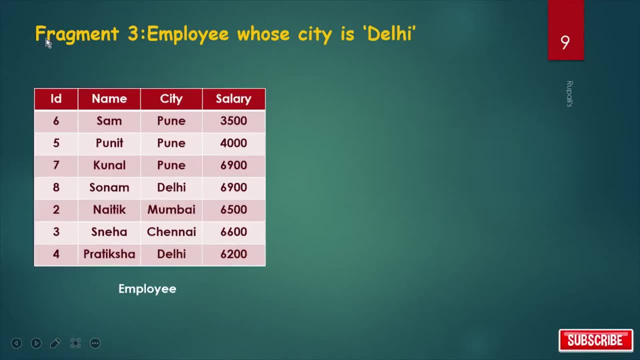 should be create table fragment two as select star from employee where city equals to mumbai. and fragment two is like this: and for fragment three i have to select those employee whose city is delhi, so query should be: create table fragment three as select star from employee where city equals to delhi, so fragment. 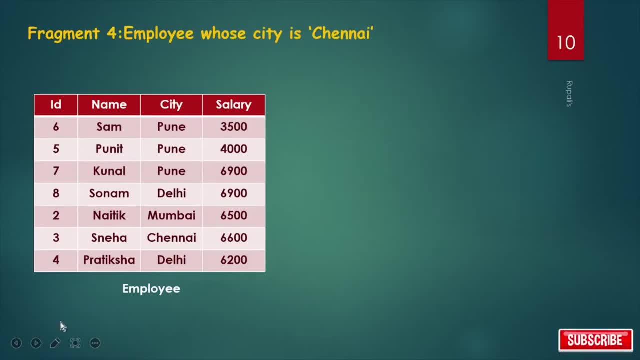 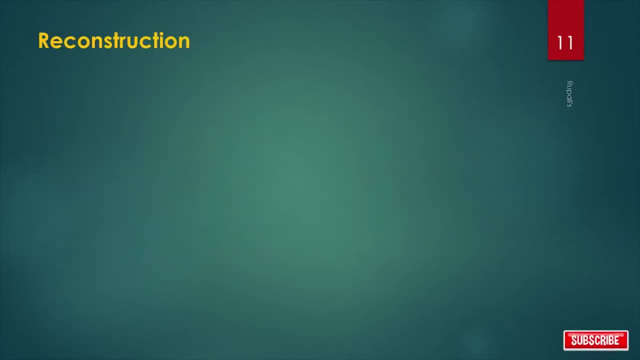 three will be looked like this. fragment four is we have to select those employee whose city is chennai, so the query should be create table fragment four as select star from employee where city equals to chennai. and fragment four will be look like this: now we can reconstruct. 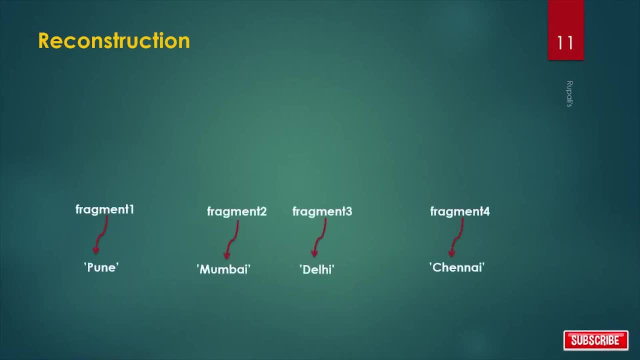 the original table from those fragments. so fragment one based on city pune, fragment two based on city mumbai, fragment three based on city delhi and fragment four based on city chennai, we have to do union between first two fragments and another union between second two fragments means for fragment three and fragment four we have to do one. 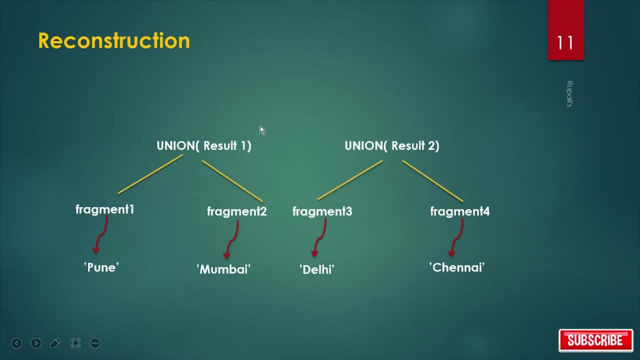 union and for fragment one and fragment two we have to do another union. we get result one and result two. again from those result we give another union to get the final result. so for reconstruction we need union. if it is horizontal fragmented table, then for reconstruction and to get the original table we have to do union correctness, rules of fragmentation, why? 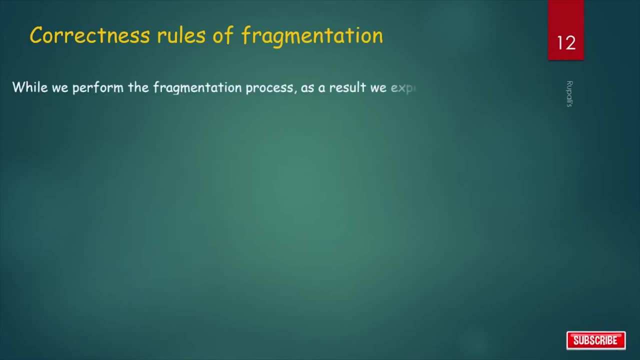 correctness rules are required in case of fragmentation. while performing fragmentation process, we should aware of these two facts. first one is: we should not lose data because of fragmentation. fragmentation means the whole table is divided into sub tables and we have to spread those table in different sides. now there should be some chance. 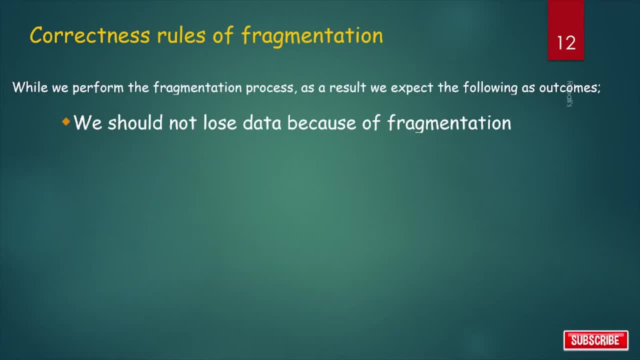 to lose data, but in case of fragmentation we should avoid that. we should not lose data because of fragmentation. and second one is we should not get redundant data, because of fragmentation means after joining again fragmented parts. if i want to join those fragmented parts and get the original table, there should be some redundant data, but we should ever. 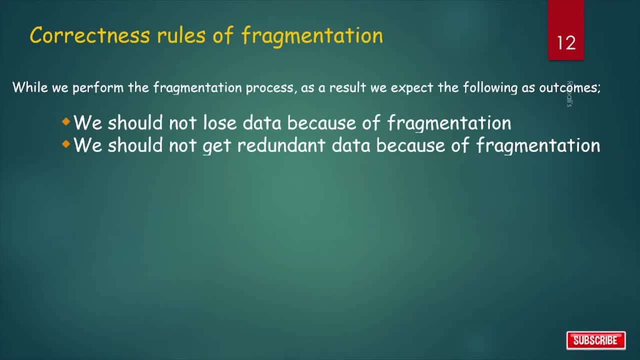 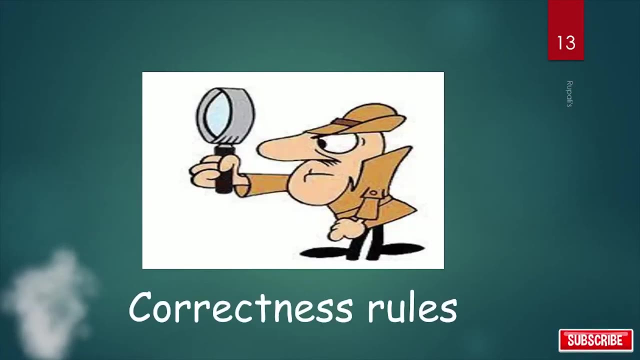 for this fact that we should not get any redundant data because of fragmentation. hence, to ensure these properties, we need to verify that, whether we perform the fragmentation correctly or not. for this verification we need correctness rule. now we have to learn what are those correctness rules for fragmentation. so the rules: first one is completeness: completeness properties. 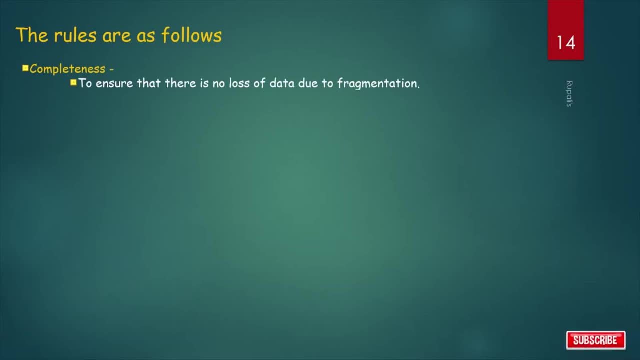 ensure that there is no loss of data due to fragmentation. it also ensures these by checking whether all the records which were part of the table before fragmentation are found in at least one of the fragments after fragmentation. reconstruction. these rules ensures that the ability to reconstruct the original table from the fragments that are created. it also ensures that 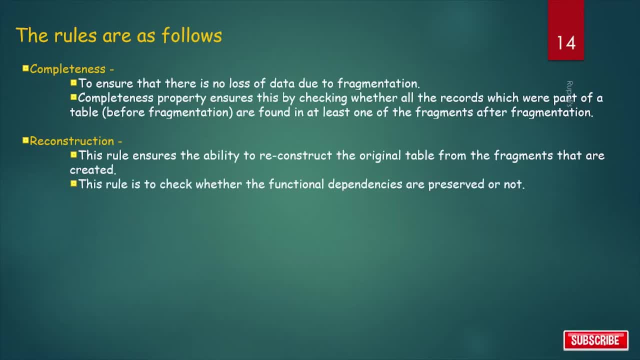 whether the function is correct or not, functional dependencies are preserved or not, and also if the whole table is R and if it is partitioned into different fragments- R1,, R2, Rn- then how we can reconstruct it. in this way, R is equals to R1, union, R2, union, R3, in this way, union Rn. and the last rule is disjointness. 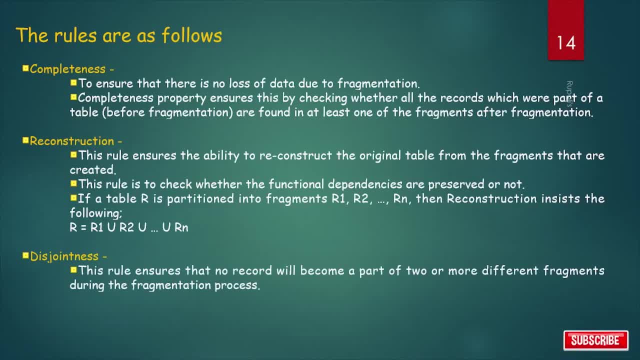 This rule ensures that no record will become a part of two or more different fragments during the fragmentation process. If a table R, say, partitioned into different fragments R1, R2, Rn, then disjointness insists that if R1 intersection R2 intersection R3, in this way: 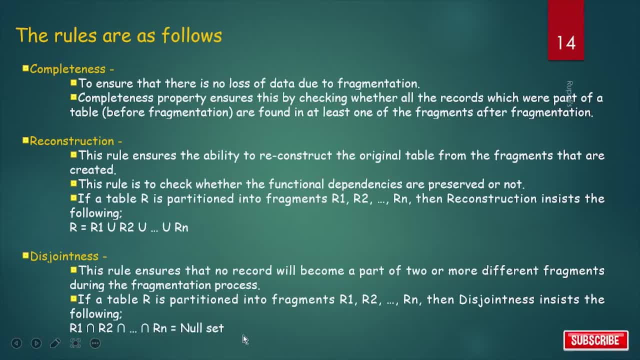 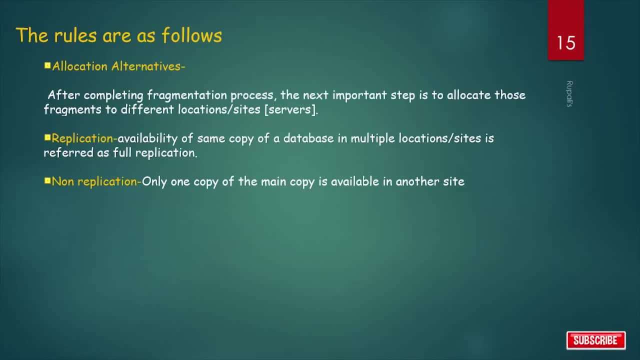 intersection Rn it should be null set that there is no redundancy Allocation alternatives. After completing fragmentation process, the next important step is to allocate those fragmentation processes. So, for example, if a table R is partitioned into different fragments, those fragments to different locations or sites, that is, in different server. 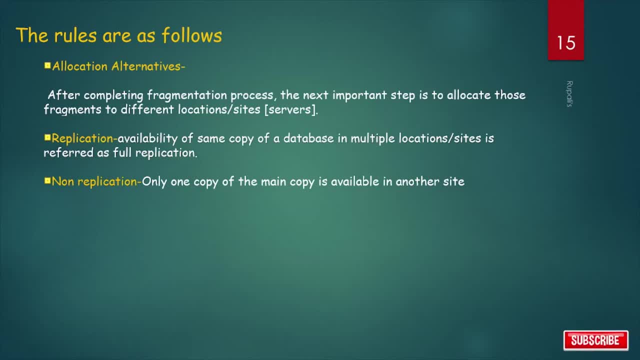 Second one is replication. What is replication? Availability of the same copy of database in multiple location or site is referred to as full replication, And what is non-replication? If only one copy of the main copy is available in another site, then that is called non-replication. 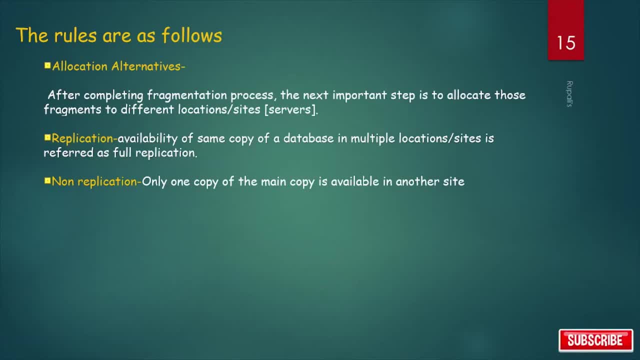 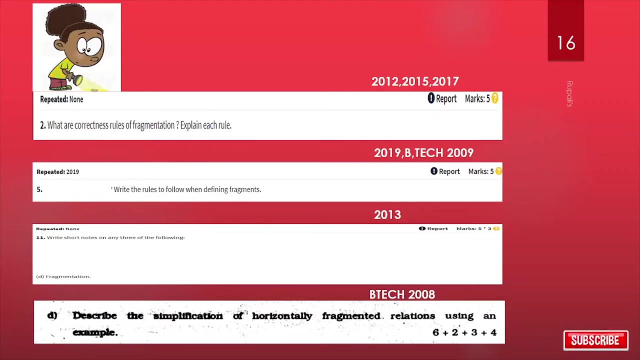 Means. there is one single copy of the original table and that is stored in another site and no other site. get the replicated copy, Only one site. get the replicated copy. then that is called non-replication Types of questions. comes in your university exam. Go through this question. 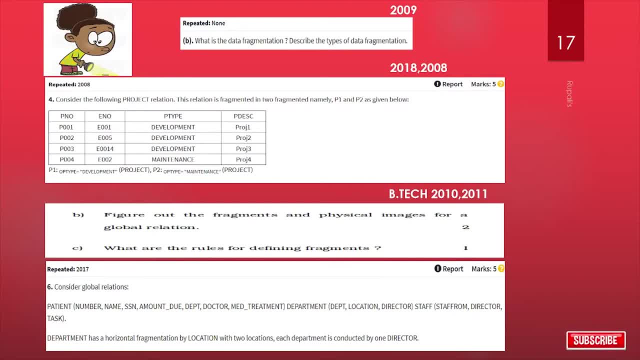 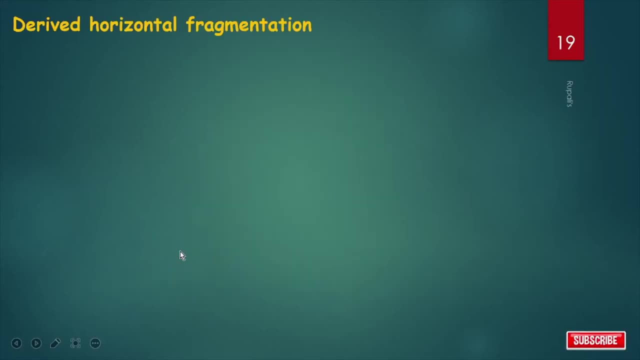 Our next topic is derived horizontal fragmentation. In derived horizontal fragmentation, a relation R1 may get fragmented by attributes of some other relation- R2.. Relation in a derived horizontal fragmentation is a relation of some other relation are classified in this way: There is one owner relation and owner relation has a primary key. 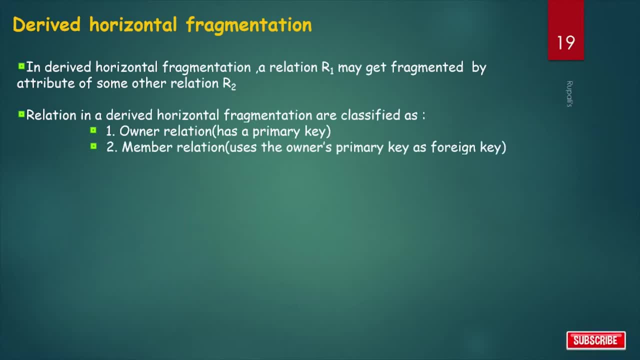 and member relation which uses the owner's primary key as a foreign key. Take one example, then this thing will be more clear for you. If, say, owner relation is R1 and the attributes are employee ID, employee name and employee salary, and employee ID is the primary key for R1 relation. 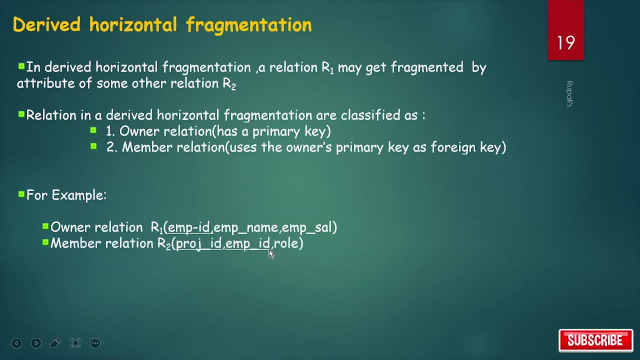 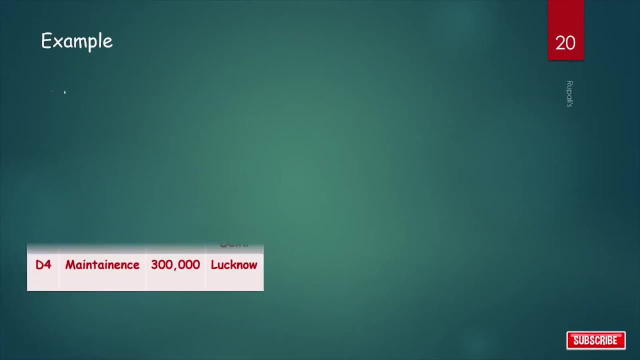 Then in member relation, employee ID is the foreign key. There is another relation, R2, and the attributes are project ID, employee ID and role. Here project ID is the primary key and employee ID is the foreign key. Take one example again. See, there is one table, department table. 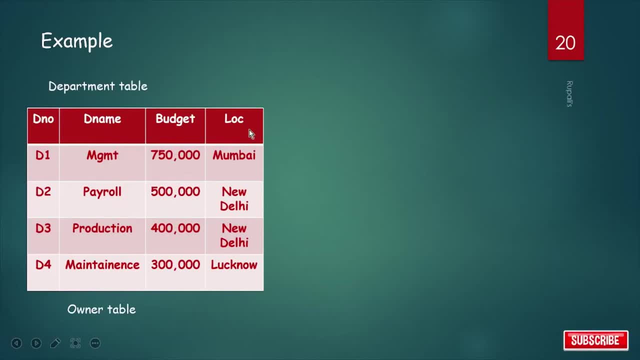 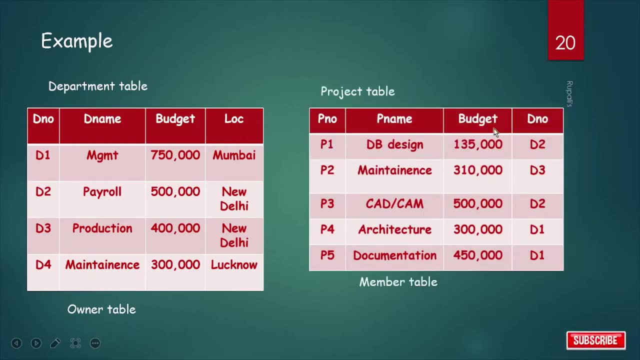 and the attributes are department number, department name, budget and location. This is owner table and the member table is project table and the attributes are PNO, PNAME, budget and DNO. See here primary key is DNO, here primary key is PNO and here DNO is the. 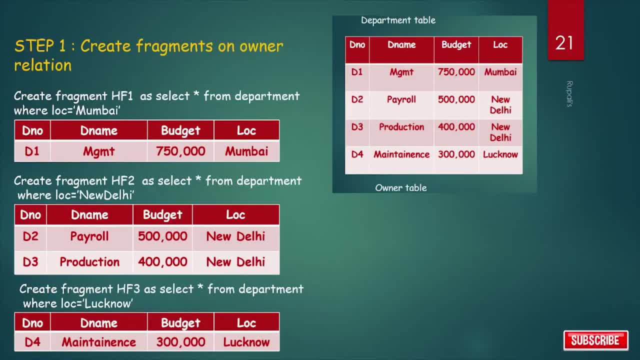 foreign key for member table. Step one: create fragments on owner relation. So this is our owner table. So first query is: create fragment HF1.. This fragment is HF1 as select star from department where location equals to Mumbai. So this is fragment HF1.. In this way create fragment. 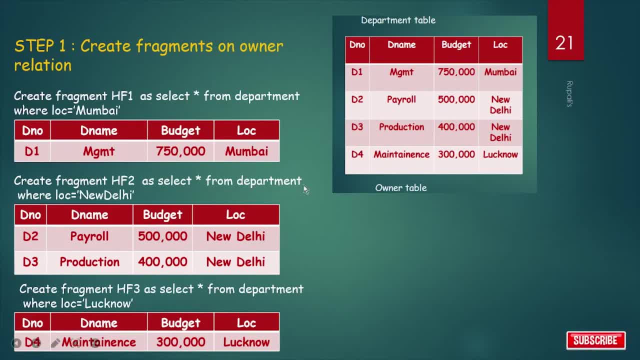 HF2.. This is fragment HF2 as select star from department where location equals to New Delhi. In the same way, create fragment HF3.. This is HF3 as select star from department where location equals to Lucknow. In this way, we can create fragments HF1, HF2 and HF3.. 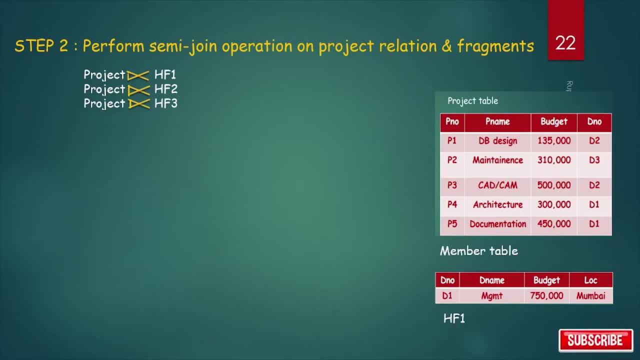 Step two: perform semi-join operation on project relation and fragments. So this is our project table, This is member table and I am taking first fragment HF1.. So first what we have to do, Let us look this up here: project semi-join HF1.. Project semi-join HF2 and project semi-join. 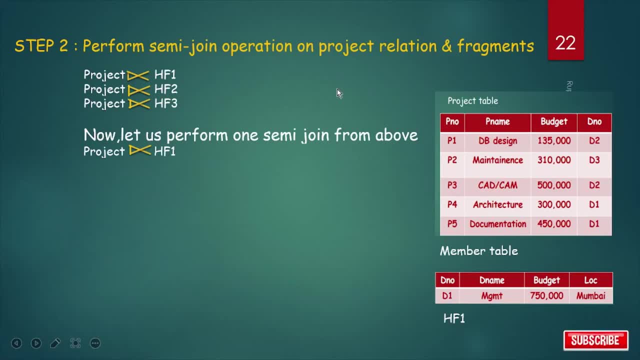 HF3.. So let us perform one semi-join from the above project semi-join HF1.. So the output should be this: This table is safe. name is project one. So after semi-join operation with HF1 and member table, we get this output. So what should be the query? So the SQL query: 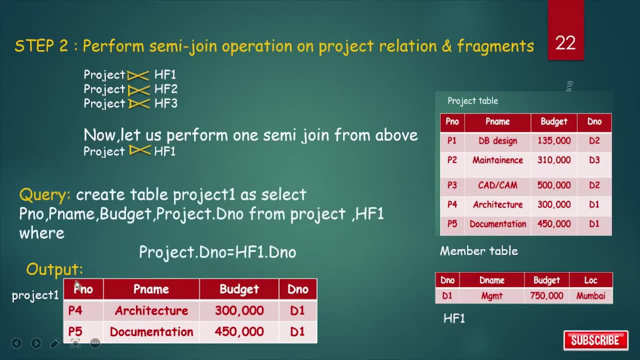 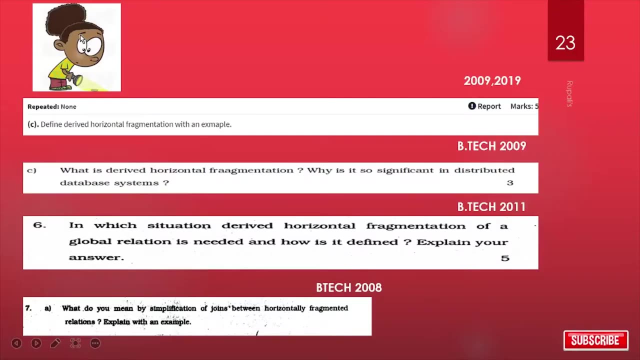 The SQL query should be like this: create table project1. this is table project1. add select pno. pname budgetdno from project and from hf1 where projectdno equals to hf1.dno. see the types of questions comes in your university exam. 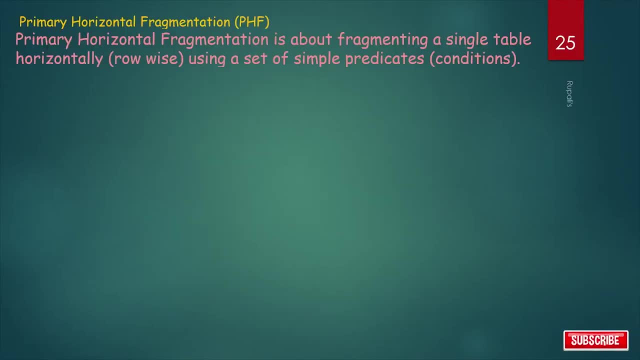 Our next topic is mean term predicate. before learning simple predicate, let's recall what is primary horizontal fragmentation. primary horizontal fragmentation is about fragmenting a single table horizontally, that is, row wise, Using a set of simple predicates or some conditions. so what is the definition of simple? 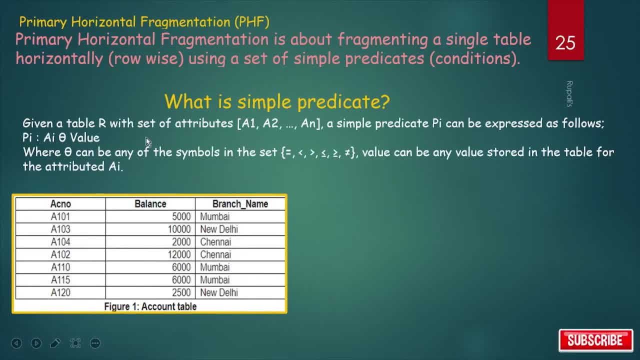 predicate: Given a table R with a set of attributes- a1, a2, an- a simple predicate, pi, can be expressed in this way: pi, colon, ai. theta value where theta can be any of the symbol in the set, that is, is: equals to less than greater than less than equals to greater than equals to. 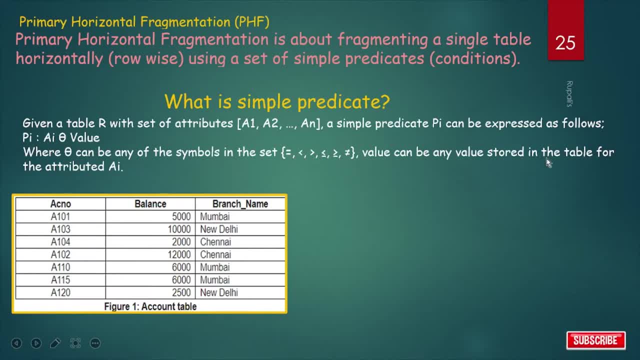 not equals to and value can be any value stored in this table, in this table for the attributes. Take one example for the table account, this table, if simple conditions are, balance less than 10000 and balance greater than equals to 10000, then set of simple predicates: p1. 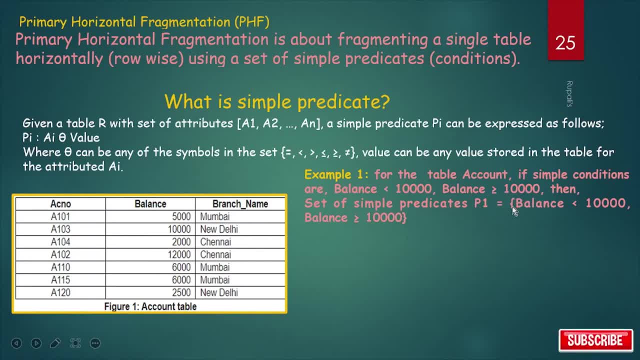 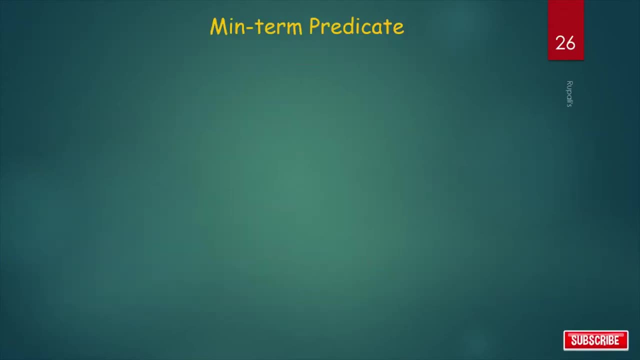 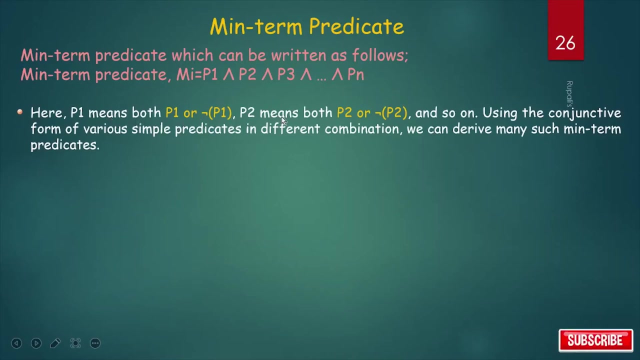 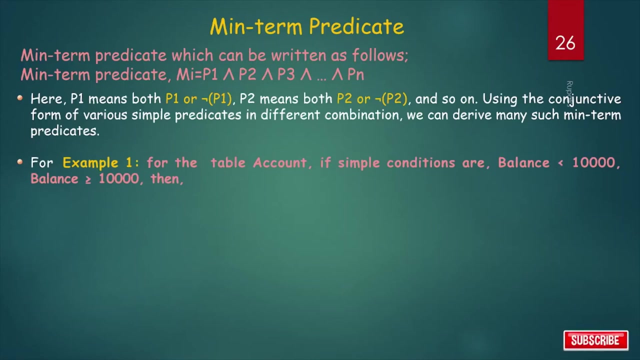 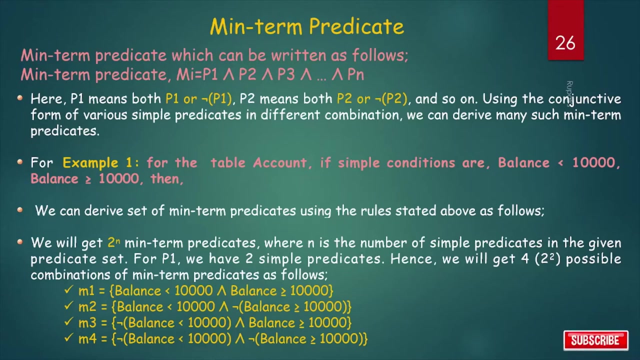 is equals to. in this way you have to write: second bracket: balance less than 10000. comma: balance greater than equals to 10000. second bracket closed. in the same way you can write also the example 2.. 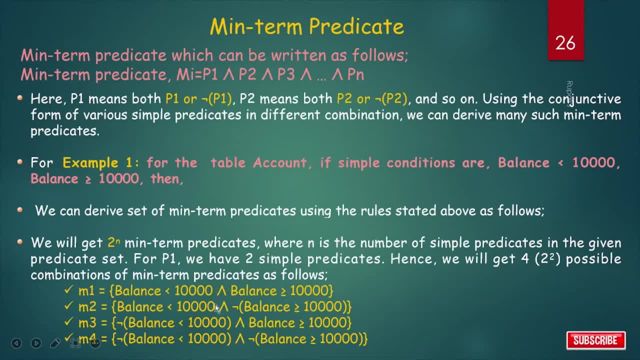 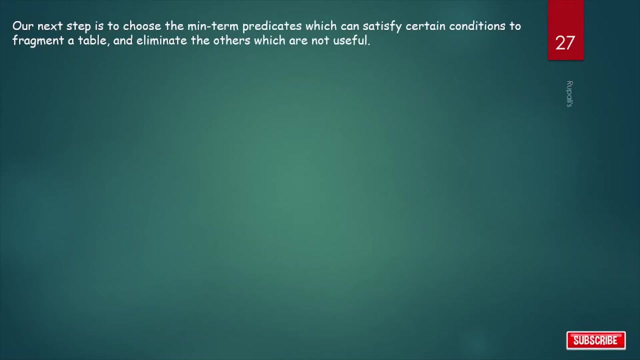 We can write the query according to the four possible combinations. So the first one is C: select star from account where balance less than 10000 and balance greater than equals. 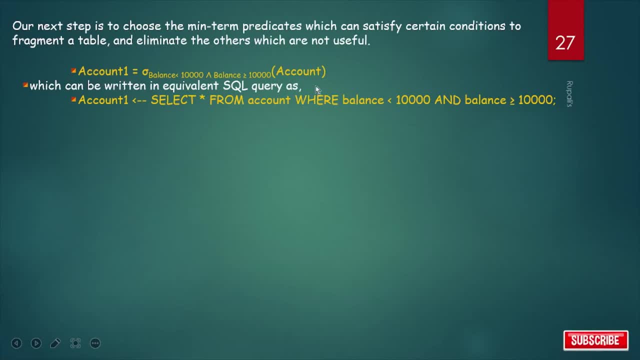 to 10000, and the relational algebra expression is this: The second one is select star from account. where balance less than 10000 and not balance greater than equals to 10000, and the relational algebra expression is this: C where not balance greater than 10000 is. 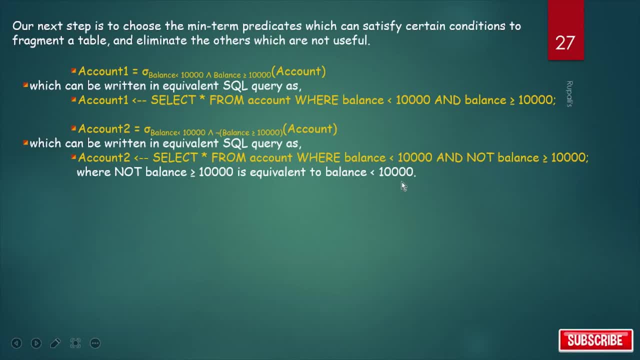 equivalent to balance less than 10000.. Combination number 3, select star from account where not balance less than 10000 and balance greater than 10000.. So the relational algebra expression is this: C where not balance less than 10000 is equivalent to balance greater than equals. 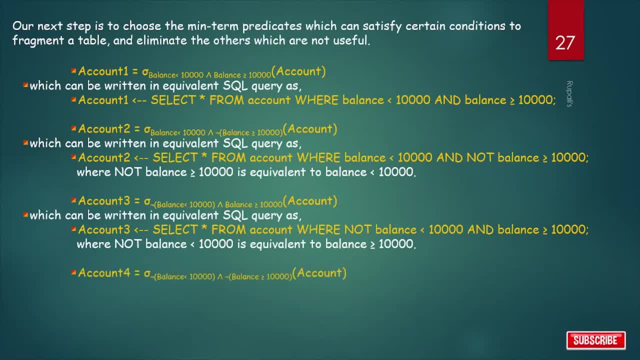 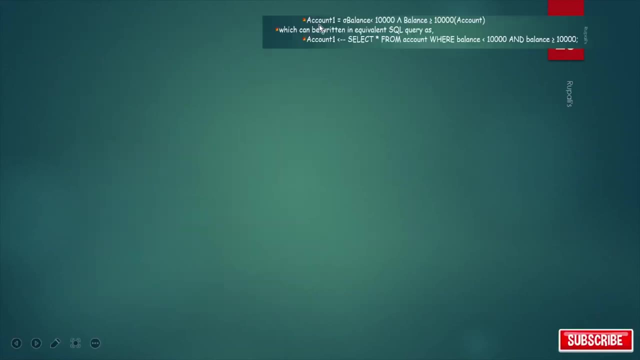 to 10000. and combination number 4, select star from account where not balance less than 10000 and not balance greater than equals to 10000.. So these are the four combinations for the first query C for account 1, for fragment account 1.. 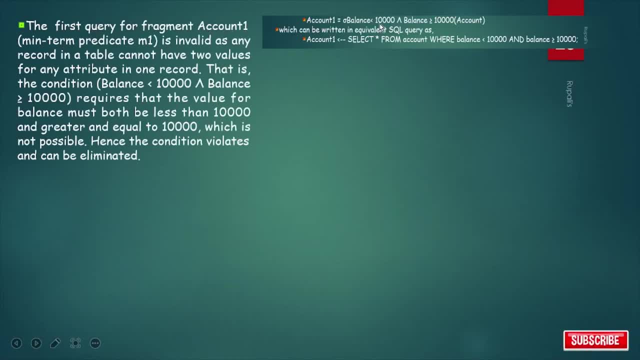 Thank You, mean term predicate is M1. it is invalid. why so? because any record in a table cannot have two values for any attribute in one record. that is see the condition. balance less than 10,000 and balance greater than equal to 10,000 requires that the value for balance must both. 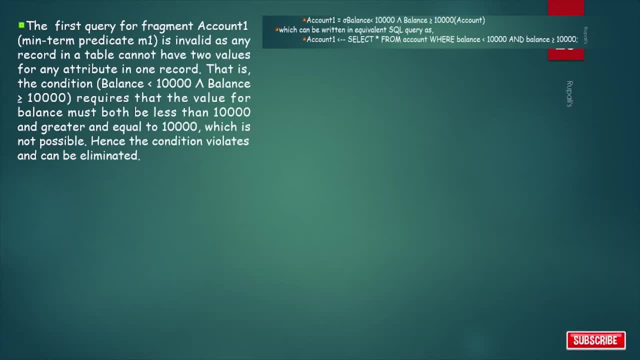 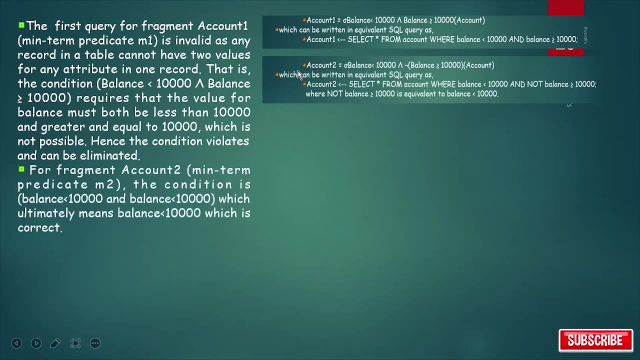 be less than 10,000 and also greater than and equal to 10,000, which is not possible. hence this condition violates and we can eliminate this condition. For the second one- this is our second query- for fragment account 2, mean term predicate is M2, see the condition here the 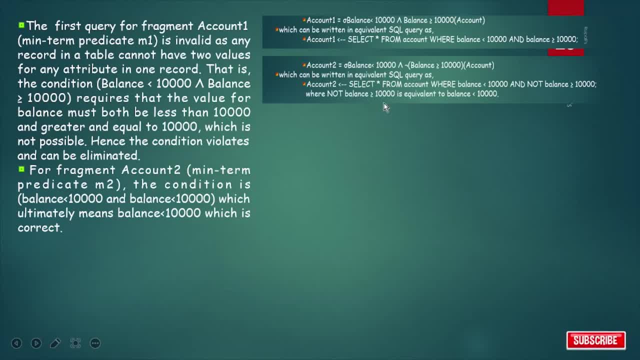 condition is not balance greater than equal to 10,000 and also balance less than 10,000, which means the condition is balance less than 10,000 and balance less than 10,000. Which ultimately means balance less than 10,000, which is correct. So the table is, which we can. 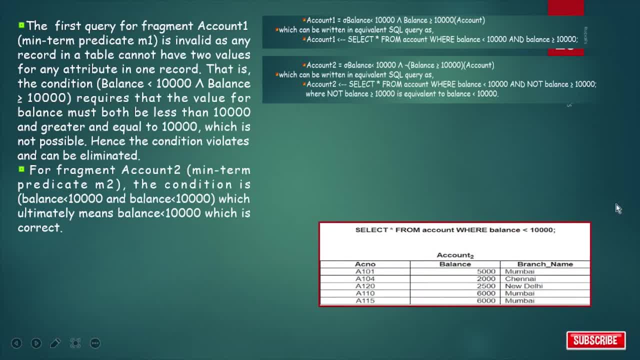 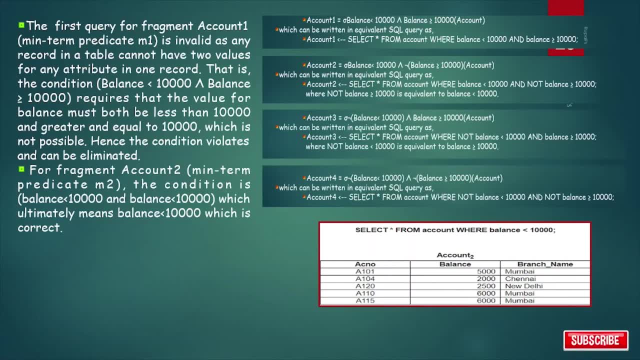 select from the account table is this: this is account 2 table Query for account 3 and account 4. for account 3, it is valid. for account 4 it is invalid. why? so? see the query where not balance less than 10,000 and balance greater than equal to 10,000 means. 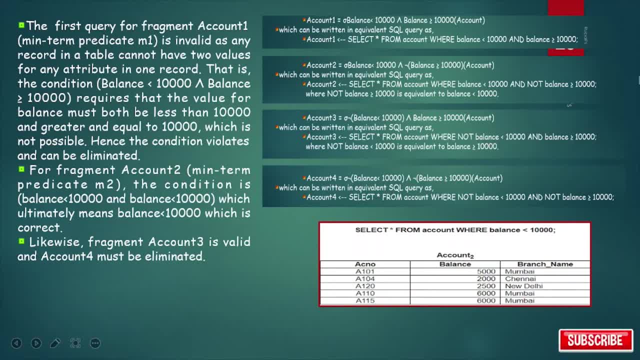 not balance less than 10,000 and balance greater than equal to 10,000.. Not balance less than 10,000 is equivalent to balance greater than 10,000. So we have to select those tuples whose balance is greater than 10,000 from the account table. So account 3 table is this: 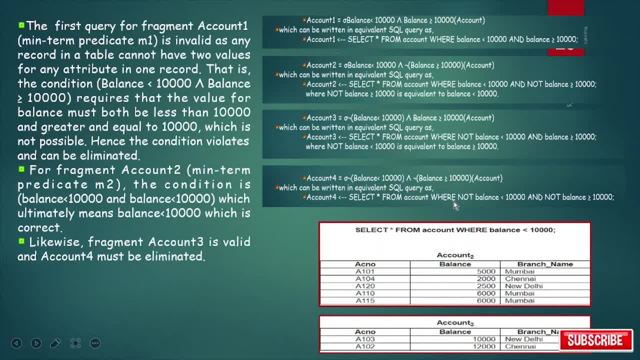 balance greater than equal to 10,000. and for account 4, see the condition where not balance less than 10,000 and not balance greater than equal to 10,000.. So which tuple? we can actually select nothing. so account 4 must be eliminated. So this is the university type question. 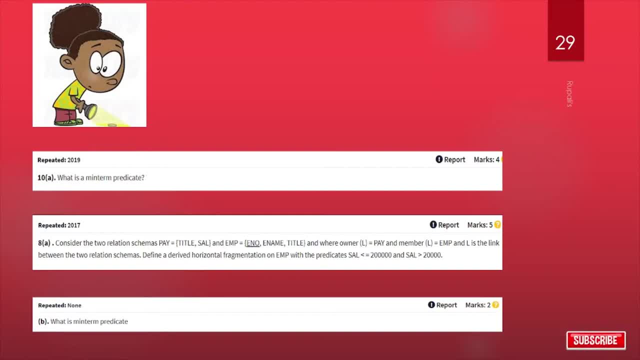 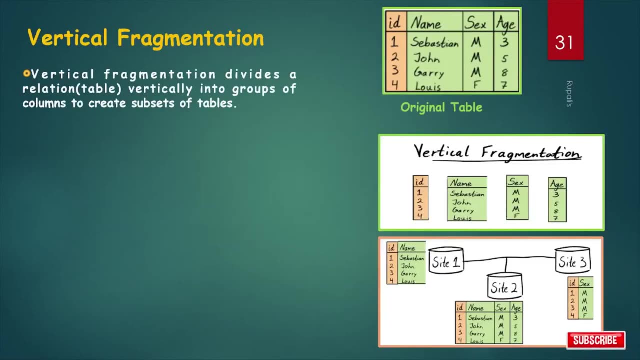 go through this question And if you are facing any problem, please write in your comment section. Our next topic is vertical fragmentation. So what is vertical fragmentation? In case of vertical fragmentation, it divides a relation or a table vertically into groups of columns to create: 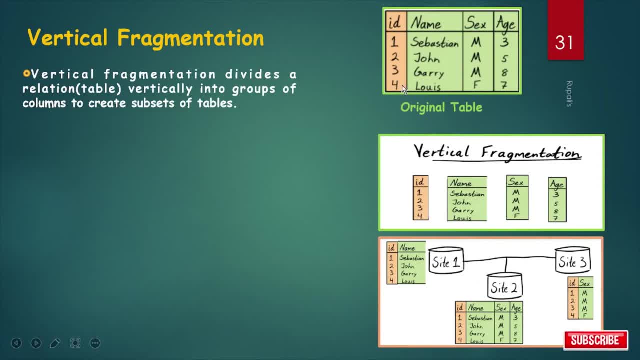 subset of tables. So this is our original tables and these are the vertically fragmented parts. Now, in vertical fragmentation the fragments are created by dividing according to their attributes. So in the original table these are the attributes: the id name, sex and age. 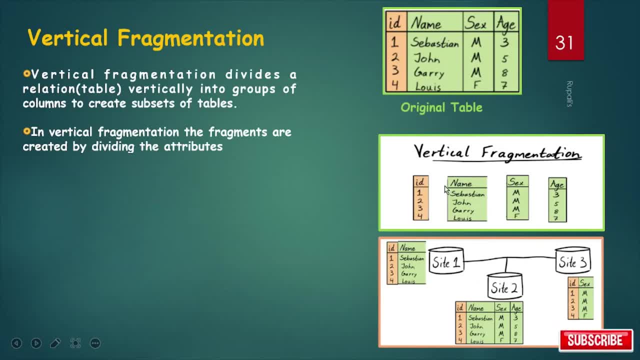 So, according to the attribute, the vertical fragmentation is done. vertical fragmentation is more complex than horizontal fragmentation. Why so? because, in order to maintain reconstructiveness, each fragment contain the primary key fields of the table. means if I want to again reconstruct the whole table and if I want to get the original table, we have to give or we have to contain primary key, what is? 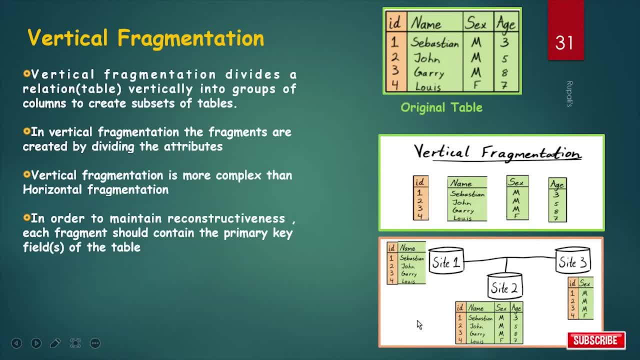 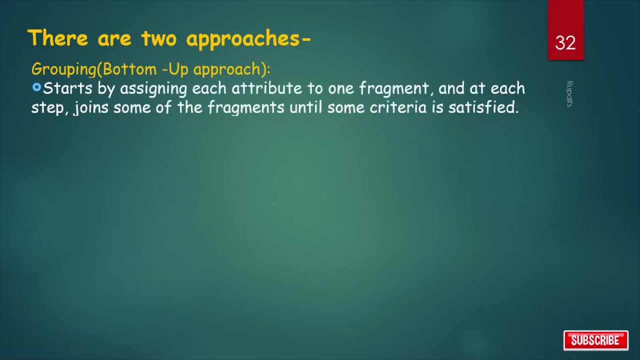 the primary key here id. so to reconstruct the original table, we have to maintain or we have to contain the primary key in each fragment. there are two approaches for vertical fragmentation. first one is grouping or bottom-up approach. in this approach we have to start by assigning each 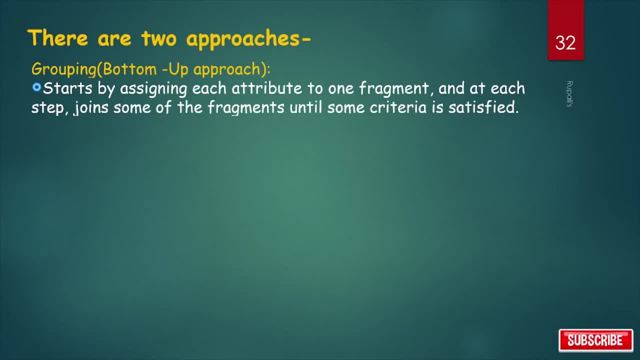 attribute to one fragment and at each step join some of the fragments until some criteria is satisfied. so each step we join two or more fragment. okay, attributes are progressively aggregated to constitute fragment. this is called bottom-up approach. another approach is splitting or top-down approach. this is just the opposite of 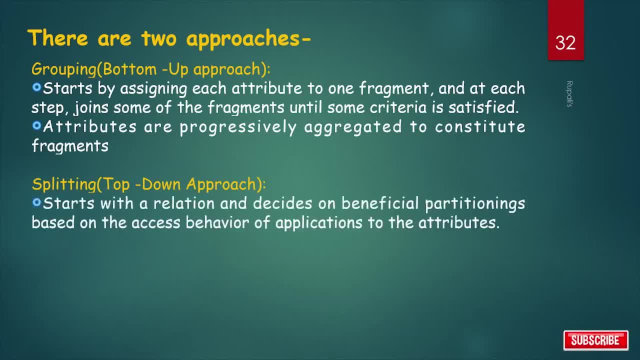 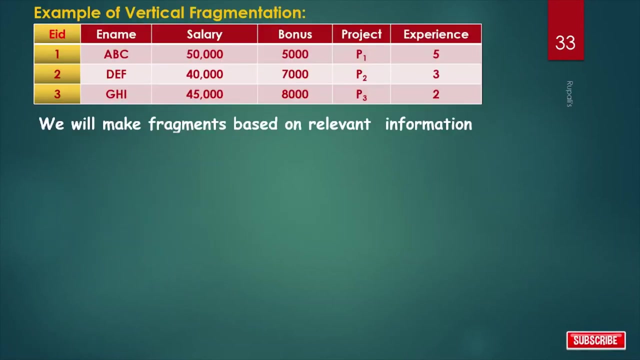 previous one. here we start with a relation and decide on beneficial partitionings based on the access behavior of application to the attributes. here global relations are progressively split into fragments, so this is called bottom-up approach and this is called top-down approach. now take one example for vertical fragmentation. here this is one employee table and these are the required. 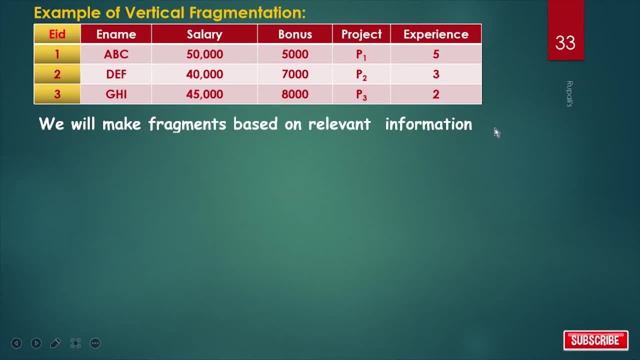 attributes and EID is the primary key for this table. Now, in case of vertical fragmentation, we already learned that we will make fragments based on the relevant information and primary key is included in every fragment. So we make two fragment: fragment 1 and fragment 2.. Fragment 1 is: it is the basic. 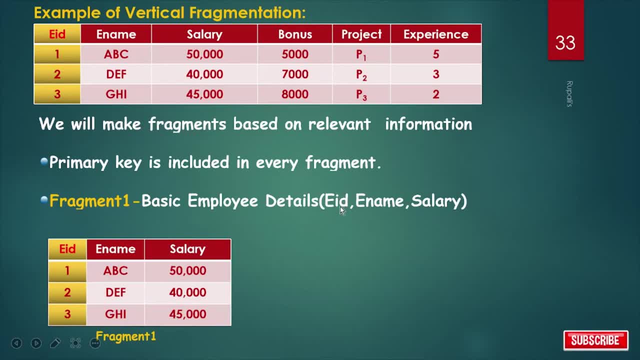 employee details. here required attributes are EID, E, name and salary. This is fragment 1 and see. EID is here. this is the primary key and for fragment 2: this is fragment 2. this is bonus on project. here the required attributes are EID, bonus and project See. for each fragment there is 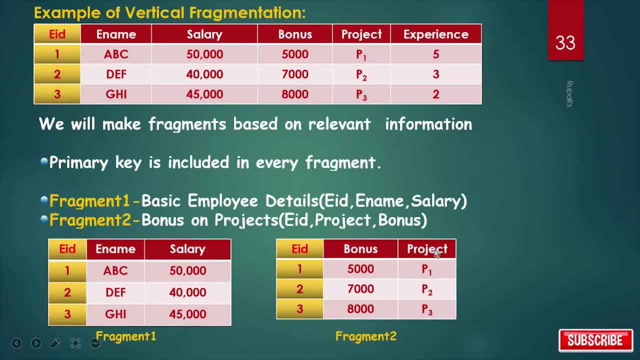 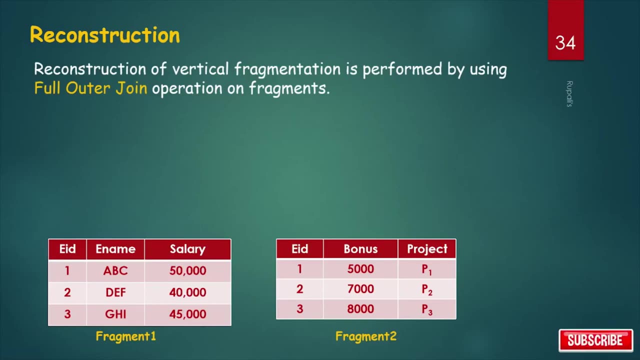 primary key. Why so? Because for reconstructiveness it is necessary. If I want to reconstruct the whole table, then this EID should be in both fragment, otherwise we cannot reconstruct the whole table. So how we can reconstruct the vertically fragmented table? Reconstruction of 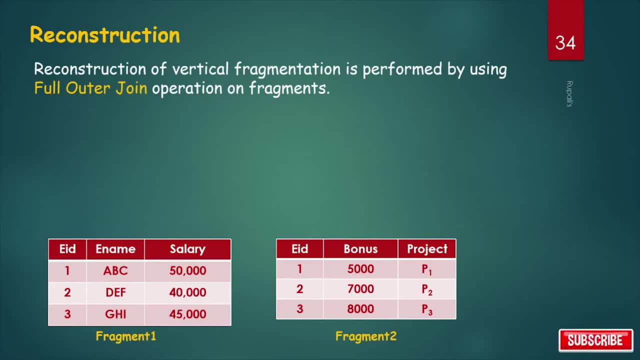 vertically. fragmentation is performed by using full outer join operation on fragments. So if this is fragment 1 and this is fragment 2, then we require full outer join operation. So the required SQL query is: select star fragment 1, natural join fragment 2.. Types of questions comes in your 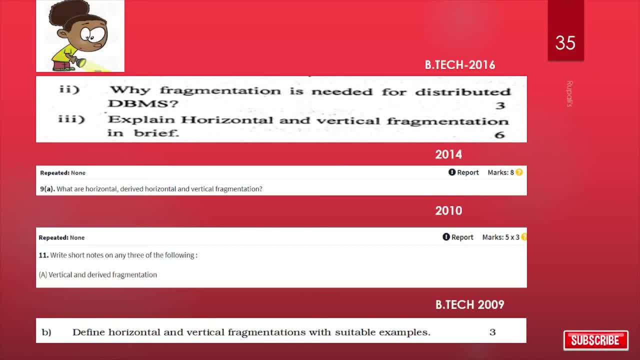 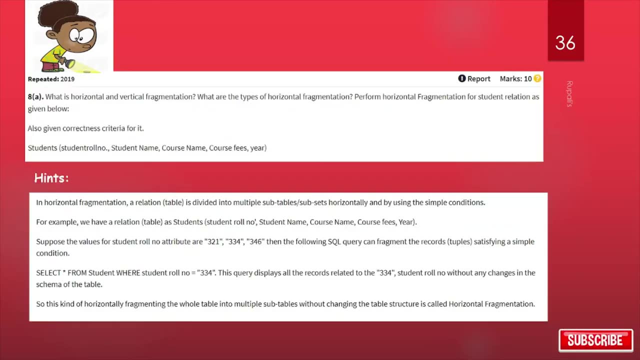 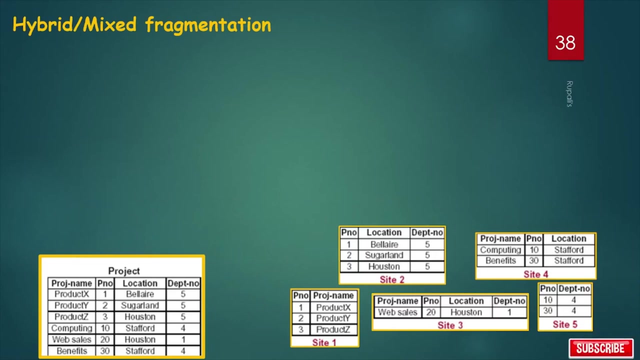 university exam. Go through this question and if you are facing any problem, please contact us. Please comment me in the comment section. Our next topic is hybrid or mixed fragmentation. So what is hybrid or mixed fragmentation? In hybrid fragmentation, we have two types of fragmentation. Hybrid fragmentation is a fragmentation. 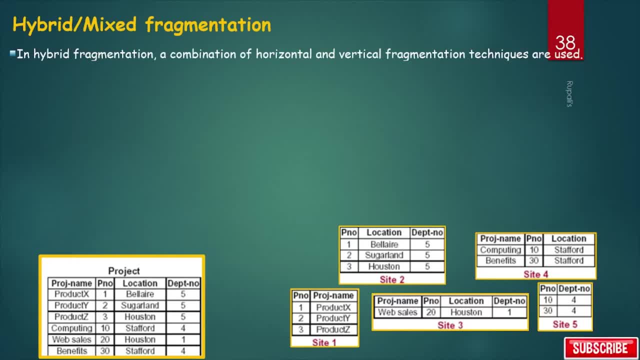 where a combination of horizontal and also vertical fragmentation techniques are used. Mixed fragmentation is a group of some rows and columns in a relation. However, reconstruction of the original table is often an expensive task because original relation is obtained by combination of joint and union both operations. Hybrid fragmentation can be done in 2 alternative. 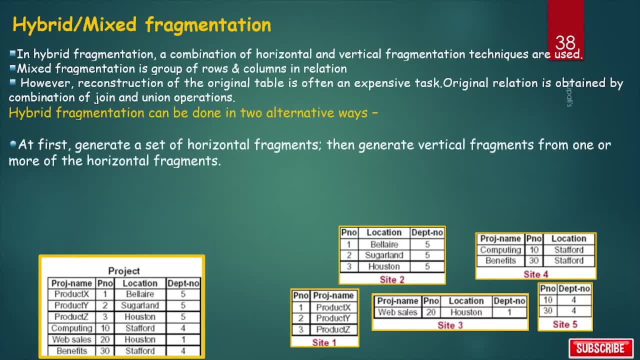 ways. one is generate a set of horizontal fragments, then generate vertical fragments from one or more of the horizontal fragments. So first you can generate horizontal fragments and from those fragments you can generate vertical fragments. and the second one is first generate a set of 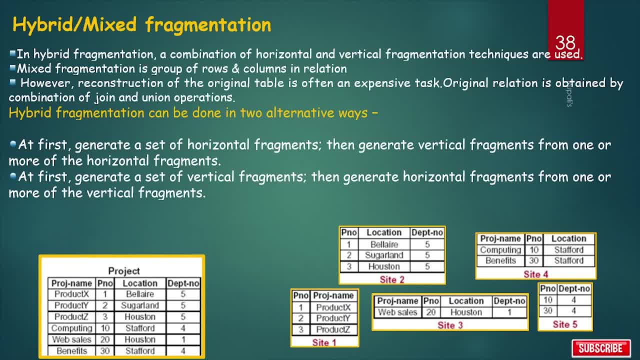 vertical fragments and then generate horizontal fragments from one or more of the vertical fragments. That is, the second one is just the opposite of the first one. So fragmentation is defined using the selection and projection operations of relational algebra. We can first project, then select, or first select and then project. Reconstruction of hybrid fragmentation. 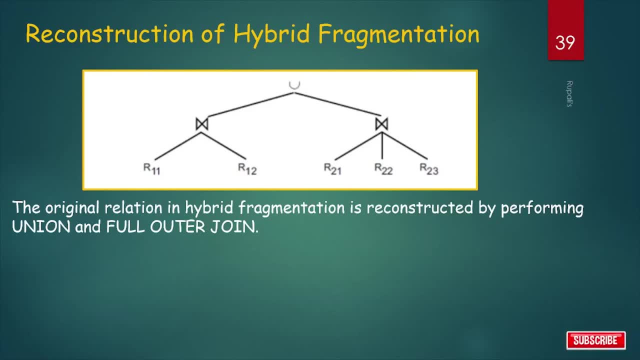 because hybrid fragmentation is the combination of both horizontal fragmentation and vertical fragmentation techniques. So if I want to get the original relation in hybrid fragmentation, it is reconstructed. So in this case, if I performing both union and full outer joint operation, because we know for horizontal fragmentation, for reconstruction of table, we need union and for vertical fragmentation- 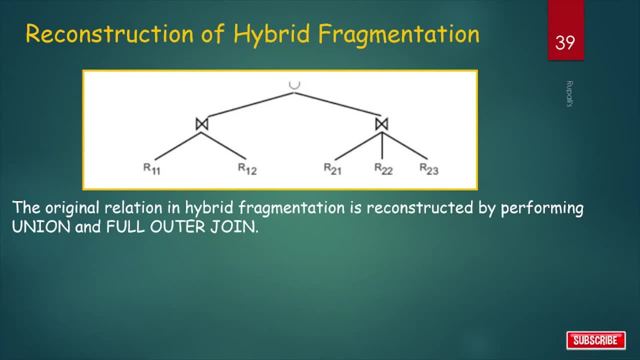 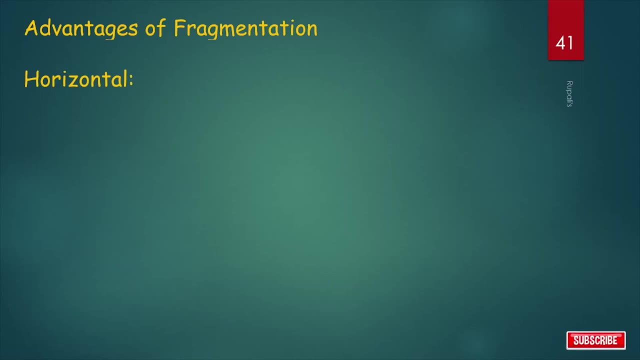 for reconstruction of table we need full outer joint operation. So for reconstruction of hybrid fragmented table we need both union and full outer joint operation. Advantages and disadvantages of fragmentation. Advantages of fragmentation: first, horizontal fragmentation. in case of horizontal fragmentation, construction method I gave some guide so we may know what. be that classification method we needed and from this concept, insertion process. So you can go ahead and add' BRAND'. So they take a few challenges for fragmentation and perform both unter joint and tore joint of typechemical xh piel market. These are the big challenges, so that you can clearly 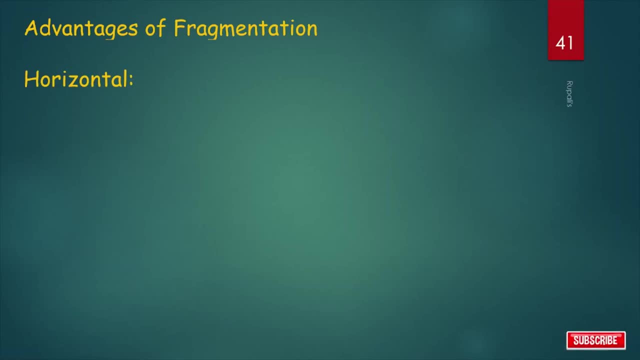 horizontal fragmentation. it is fragmented horizontally, that is, according to the row or tuples, So it allows parallel processing on fragments of a relation. It also allows a relation to be split so that the tuples are located where they are most frequently accessed, So most frequently required tuples are located at that particular site. 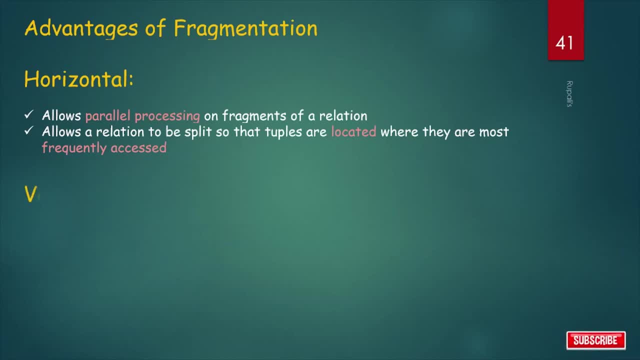 So this is the advantage of horizontal fragmentation. In case of vertical fragmentation, it also allows to be split so that each part of the tuple is stored where it is most frequently accessed, where it is most frequently required. Here, tuple id attributes allows efficient joining because primary key is in each fragment. So tuple id attributes allows efficient joining. 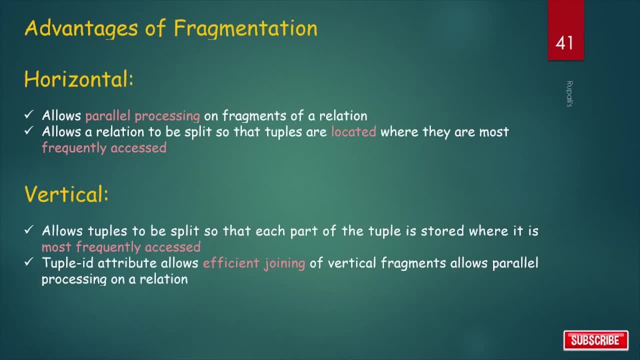 of vertical fragments, and it also allows parallel processing on a relation. So vertical and horizontal fragmentation can be mixed. that is mixed fragmentation or hybrid fragmentation. So this is the advantage of horizontal fragmentation. What is the advantage of this? Here, fragments may be successively fragmented to an arbitrary 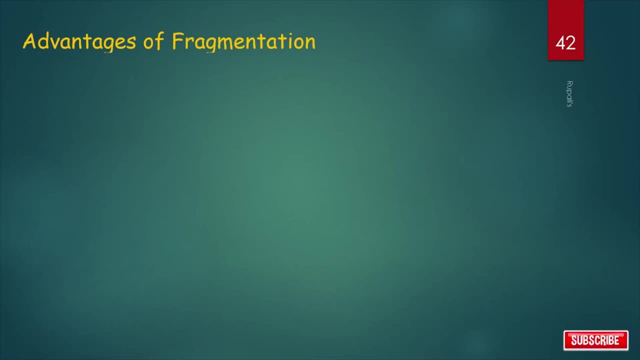 depth In an art cell. we can say that: what are the advantages of fragmentation Here? since data is stored close to the site, usage and efficiency of the database system is increased Here. local query optimization techniques are sufficient for most queries because data is locally available. 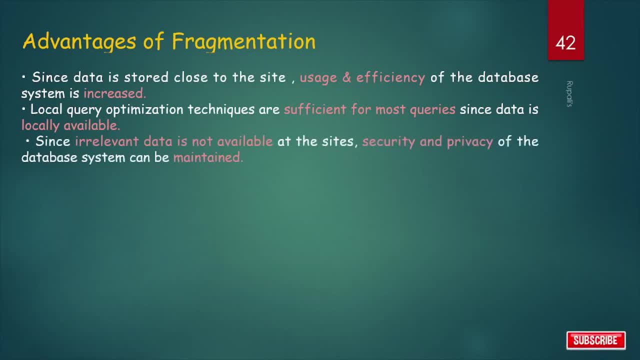 Since irrelevant data is not available at the site. so security and privacy of the database system here maintained. And the disadvantages are here when data from different fragments are required. the access speeds may be very high In case of recursive fragments, the job of reconstruction will need expensive techniques and when failure of sites occurs the data will be lost. So 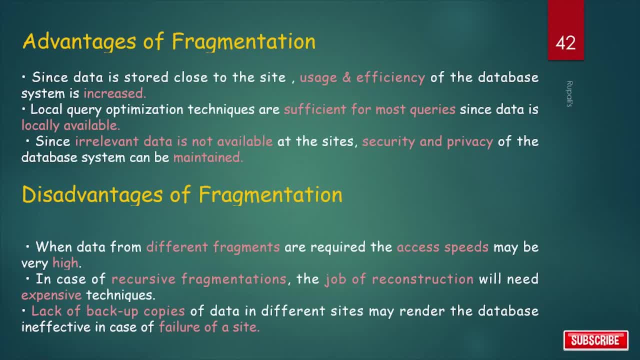 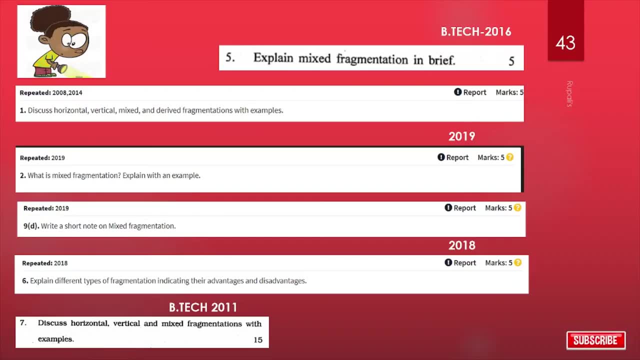 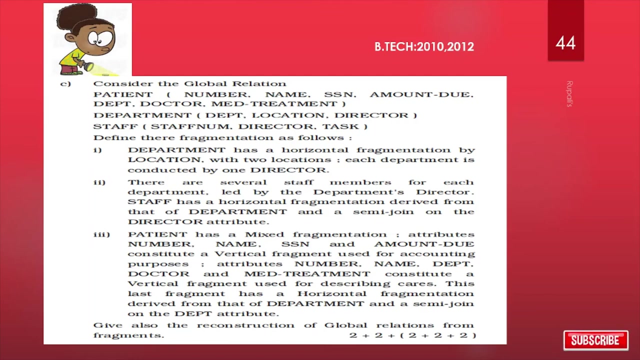 the lack of backup copies of data in different sites may render the database ineffective in case of failure of a site. See the types of questions comes in your university exam. Go through these questions For getting more and more updates on the latest developments in the database. please visit. 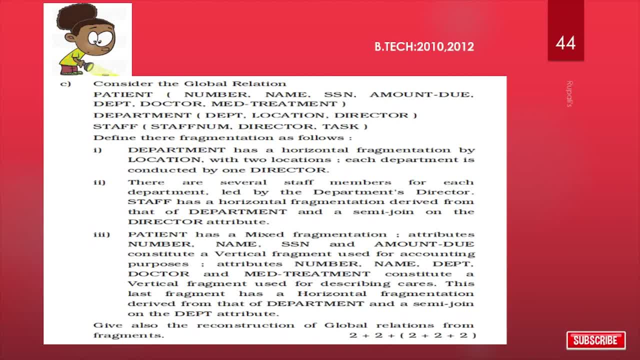 our website. Please like, share and subscribe to my channel. That's all for today, Thank you.